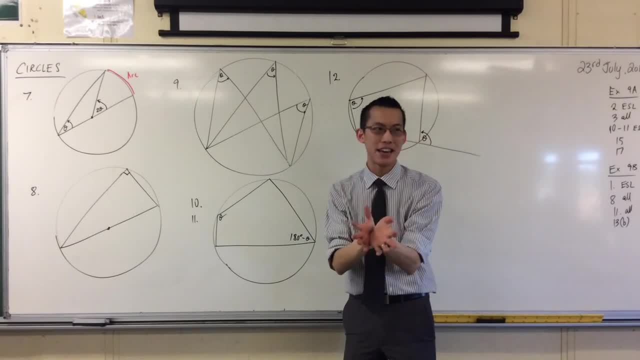 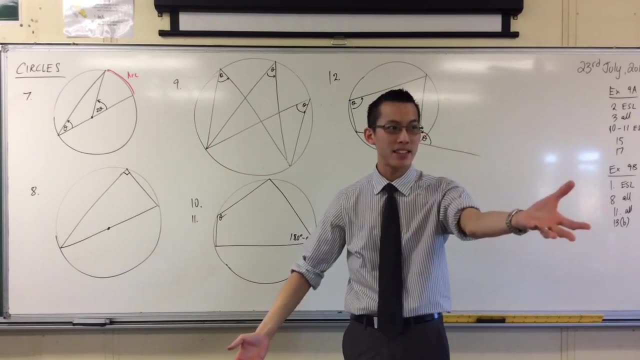 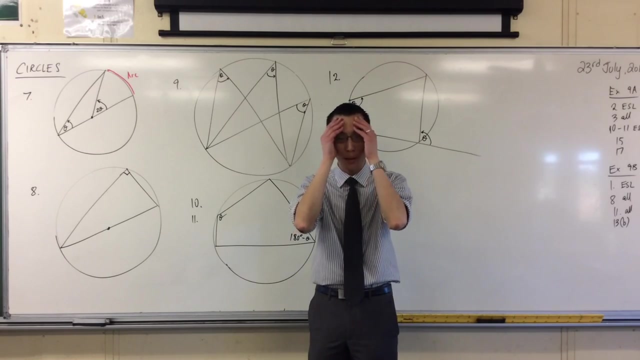 Just look at the thing: okay. In exactly the same way that in a conversation they tell you, oh, okay, if you want to get to know someone better or, like, remember their name or something like that, what you do is you say back to them, in different words, the thing they're saying to you, rather than just sort of nodding, nodding, nodding, and then five minutes later you're like: man, what were we even talking about? okay? 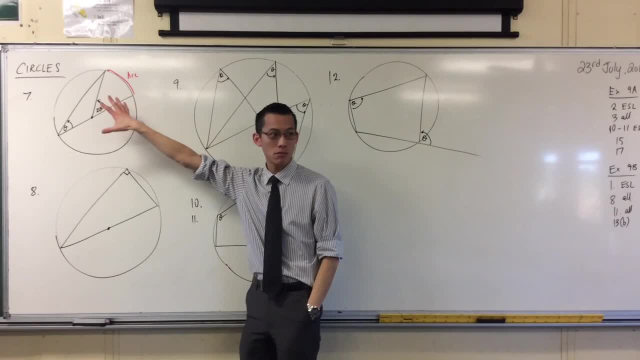 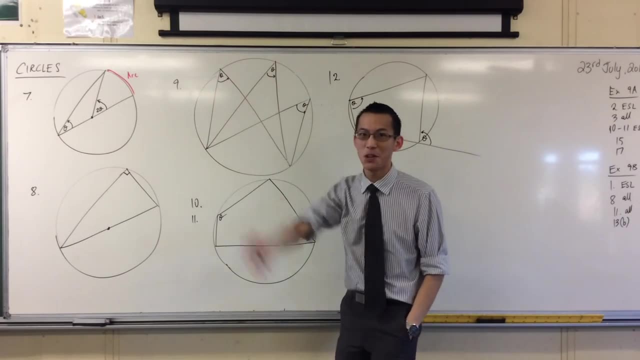 You force yourself to articulate, You force yourself to construct. okay. The other tip is- and this is why it's particularly on this one- if, after you've drawn it, it's still not clicking, turn the thing upside down. Turn the thing upside down. 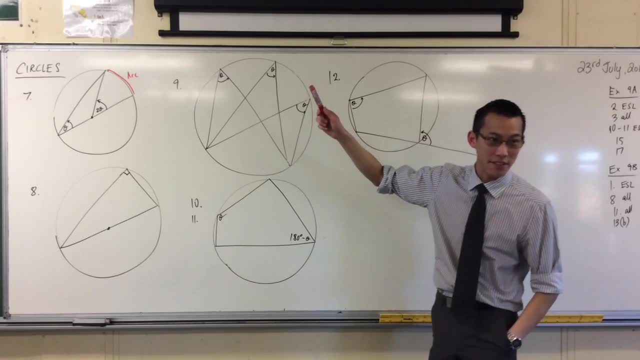 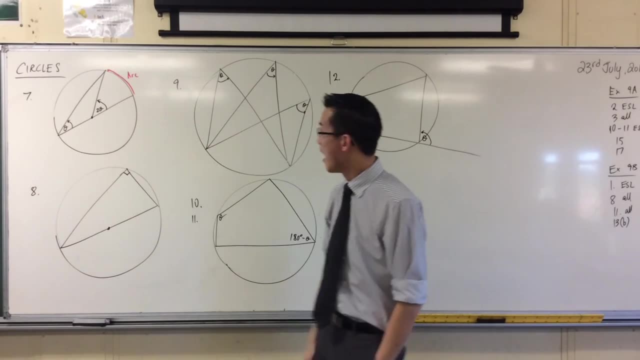 You'd be surprised- just like drawing- at how effective that kind of thing is. And it's useful here because you can't necessarily see, oh, it's standing right, because the language is not as clear, right, But if you turn it around it's pretty obvious. 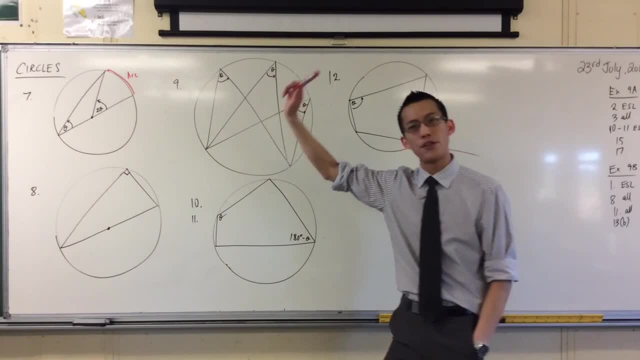 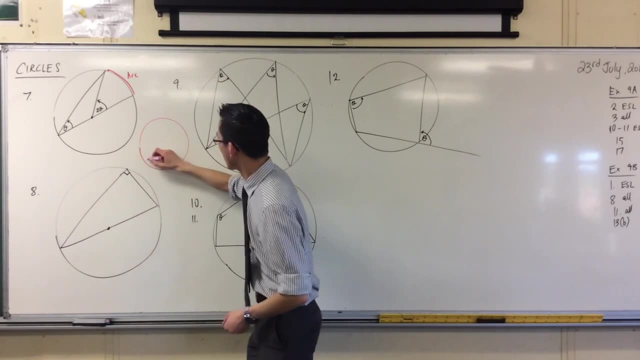 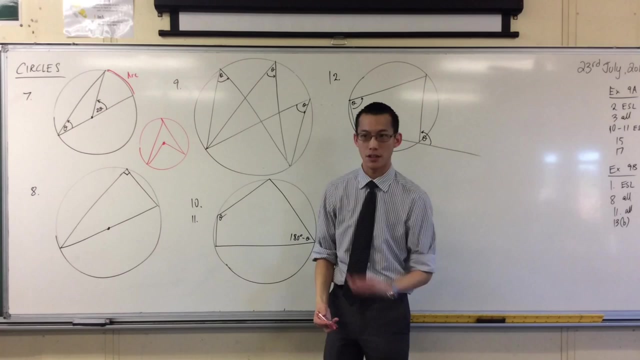 Now, how would you go about proving this? It's worth mentioning that for this particular, For this particular property, you can actually draw different diagrams to represent this. For example, here's another one: Angle at There you go. So this is the same situation, right? 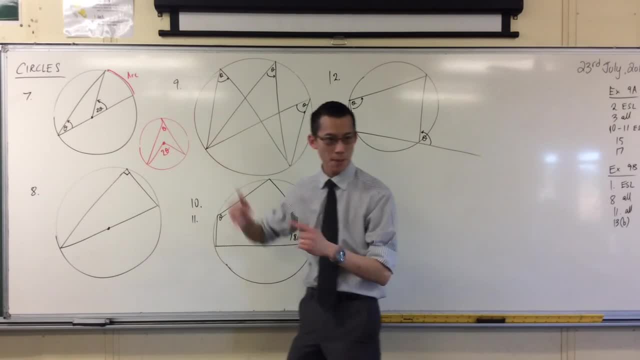 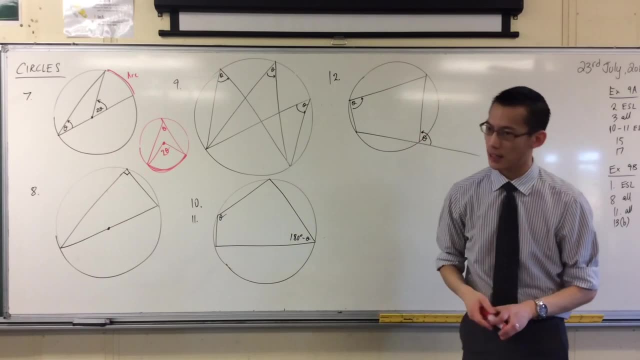 I've got an angle at the center which is double the angle at the circumference, standing on the same arc. okay, So the proof I'm about to give you doesn't quite exactly work for this, even though it works for this, because the configuration is slightly different, okay. 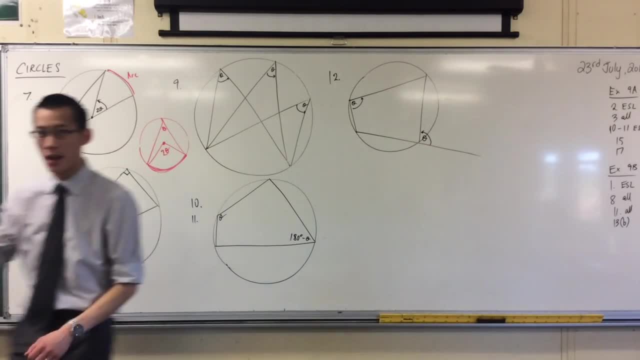 But it's not that hard. How would we construct this thing? How would we prove that these angles are the way they are? Yeah, Eddie, The triangle on the left, you prove it's an associated triangle. Okay, good. So because again we said triangles and because it's such a special triangle, you've got all these special properties. you've got radii flying everywhere, right? 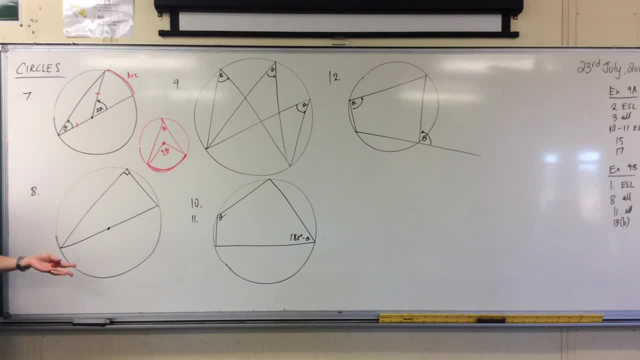 Everywhere. So therefore, as suggested, I've got that. So where do I go from there? Exterior angle: Yeah, Exterior angle, interesting sum of the Very good. So as soon as I've got, If I define that, just let that be anything you like. 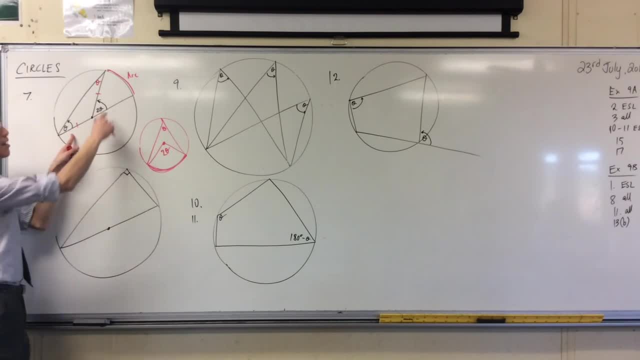 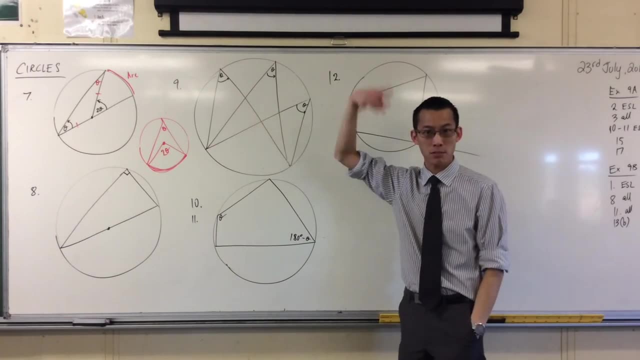 Cool, We've called it theta. That makes it theta over there because it's isosceles, And then right there, with no further constructions. the exterior angle of a triangle is equal to the sum of the opposite two interior rings, Two theta. 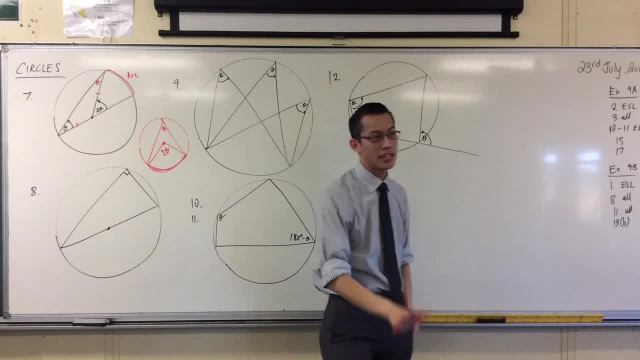 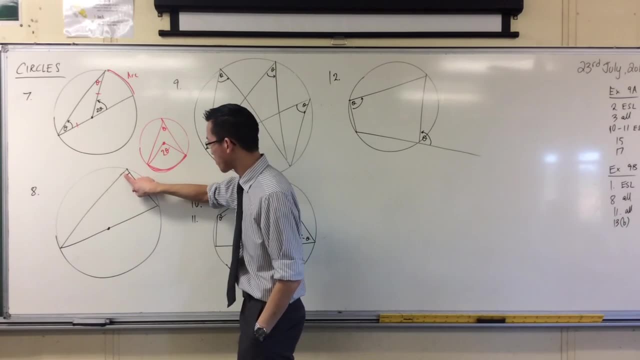 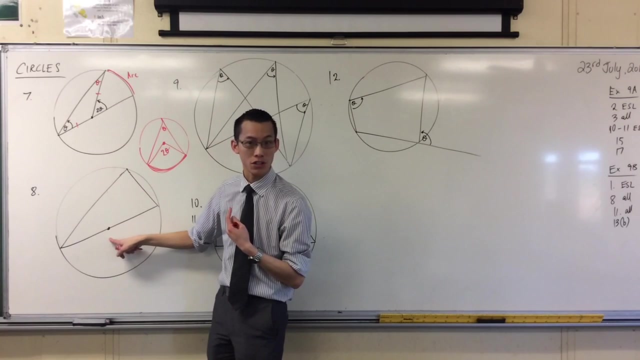 Really easy, right, When you come down to here, you're going to take advantage of another thing Because you've got the radii everywhere. you have isosceles, triangles everywhere. okay, If I wanted to prove that, this angle in the center, which I just indicate with a dot, sorry, yeah, angle in a semicircle, I just indicate the diameter with a dot there. 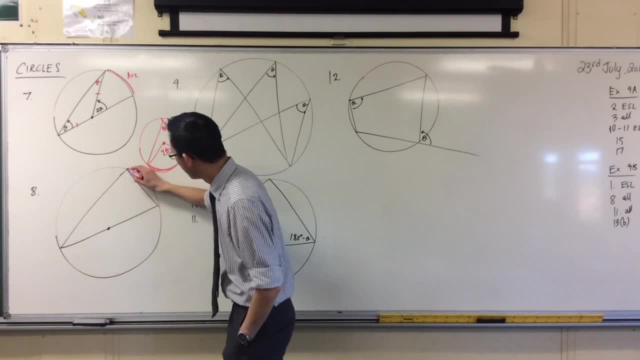 How would I do it? One line: Okay, Form the isosceles triangles right. And then what you've got here is, if I call this alpha, that's alpha right, Isosceles. you happy with that? 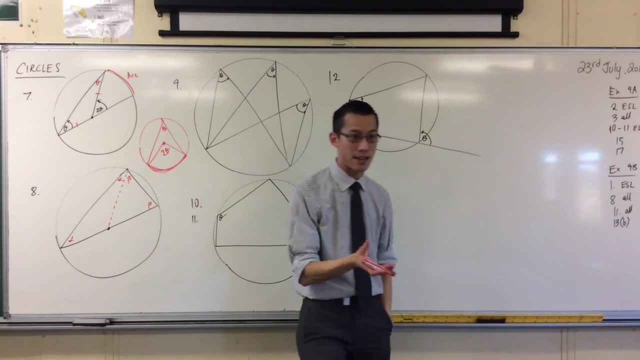 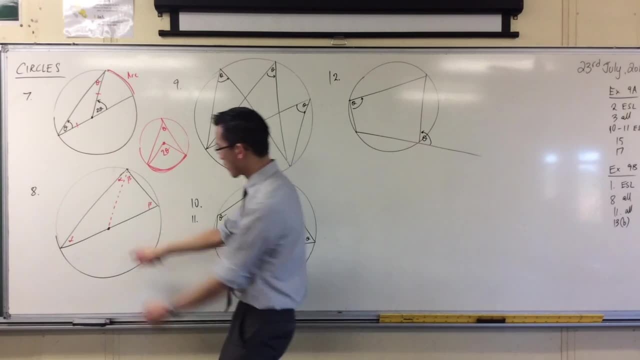 If I call this beta, I've got a beta over there, right? Because again, isosceles triangles. I'm done. Do you see it yet? What's the angle sum of a triangle? It's 180 degrees. So I've got two alpha plus two beta is 180.. 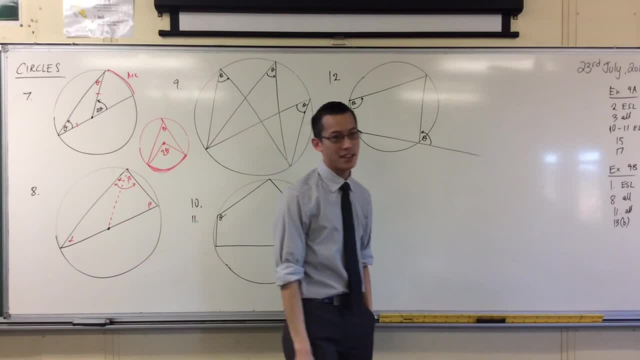 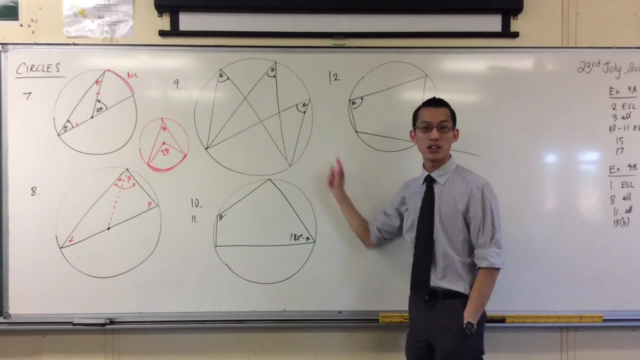 Therefore, alpha plus Beta is 90, right, Just like that. I think that's really beautiful right. Number 9 flows straight out of either of these two right. Probably 7 is the easiest right. I've got a whole bunch of angles all in the circumference. 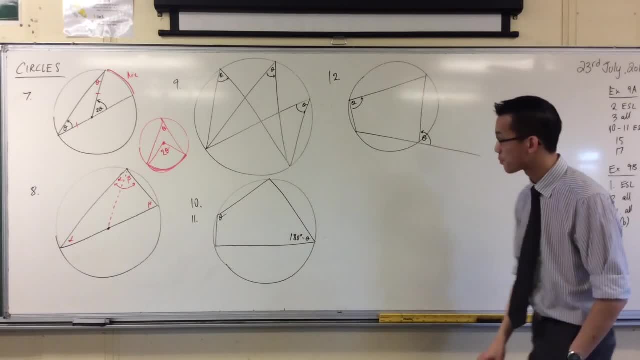 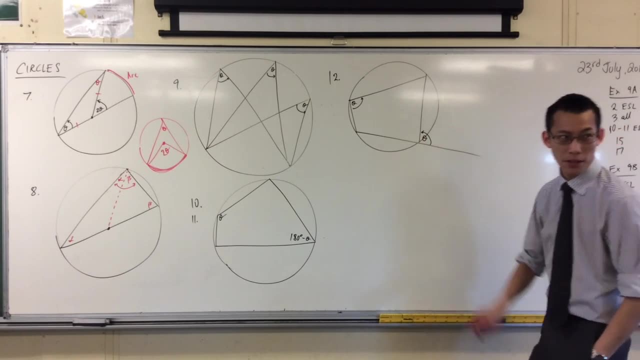 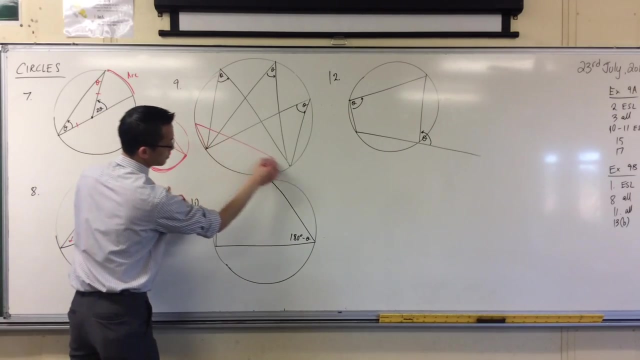 And apparently they're all equal. How would you go about showing it Now? congruence is going to be a bit tricky. Congruence will be tricky Because With these it's not obvious, But if I put one over here it's still true. 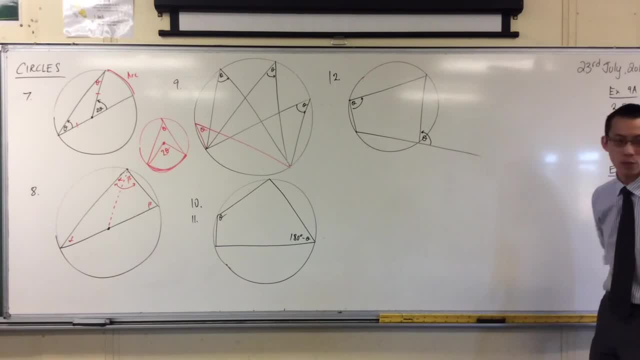 But you better believe that's not congruent, right? It's not even close to congruent. In fact, none of my original ones were congruent either. So what would you do? Where are you going to go from there, Aaron? 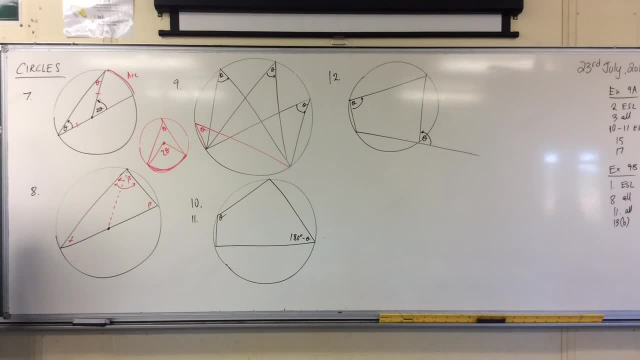 Prove all the relationship between the angle at the circumference and the angle at the center. Yeah, bingo, All right. So here we go. I've already proved this And that was easy, right? So these are all standing on the same arc, right? 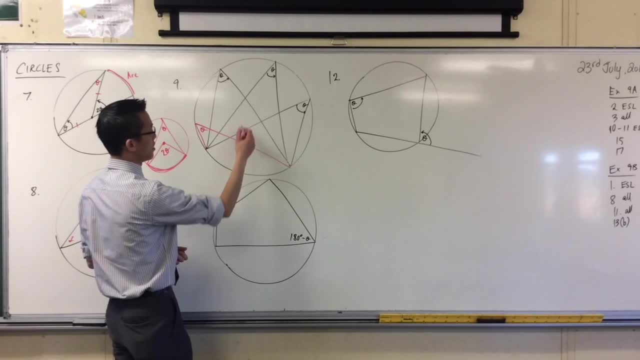 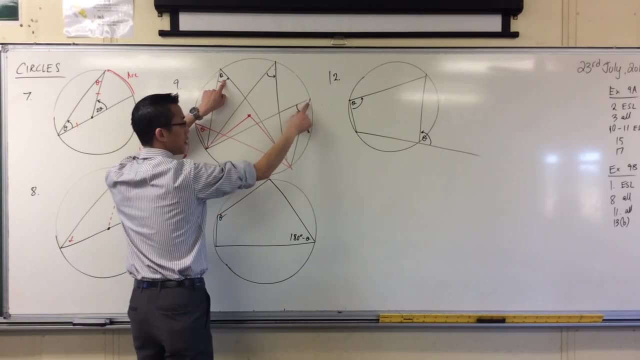 They're all on the circumference. So if I make one say here, right in the middle, If you just start from this guy and you don't know these two right, Well, this angle is at the circumference. standing on this arc down here.